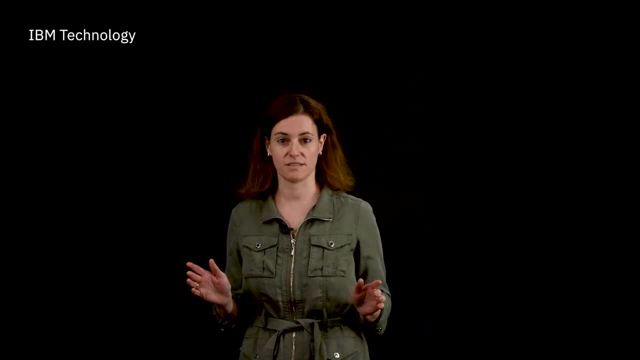 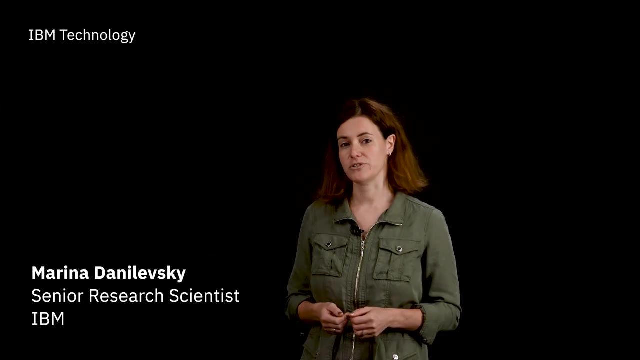 Large language models. they are everywhere. They get some things amazingly right and other things very interestingly wrong. My name is Marina Donilewski. I am a senior research scientist here at IBM Research and I want to tell you about a framework to help large language models. 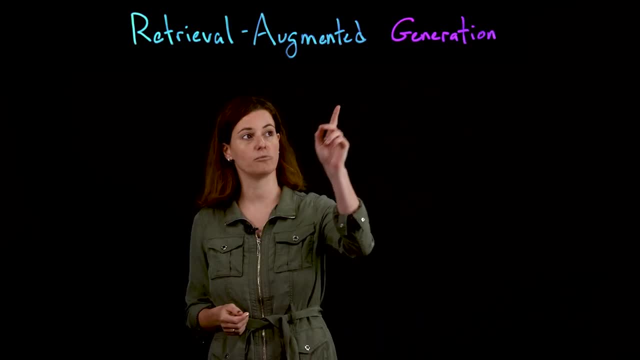 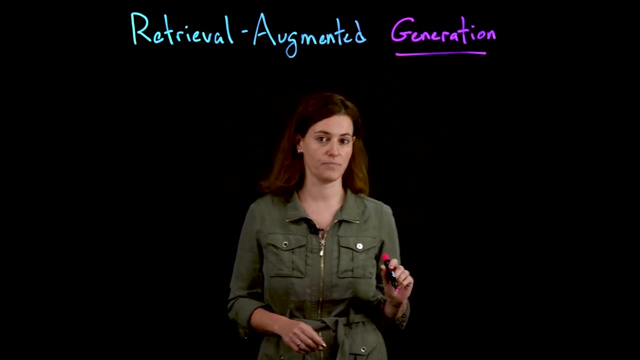 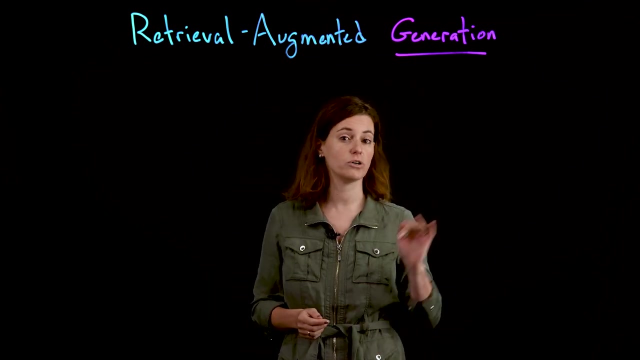 be more accurate and more up-to-date. Retrieval, Augmented Generation or RAG. Let's just talk about the generation part for a minute, So forget the retrieval augmented, So the generation. this refers to large language models, or LLMs, that generate text in response to a user query. 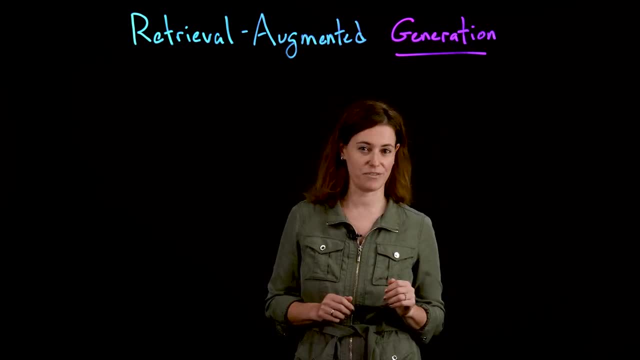 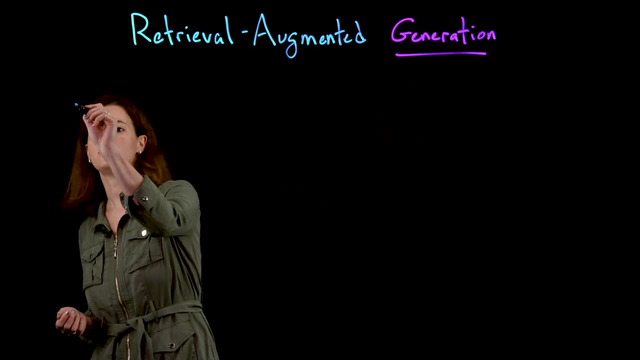 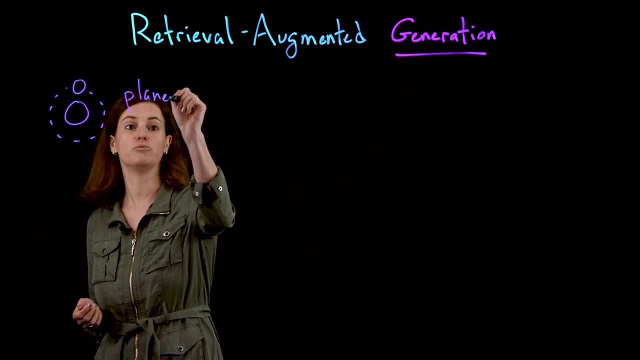 referred to as a prompt. These models can have some undesirable behavior. I want to tell you an anecdote to illustrate this. So my kids, they recently asked me this question: in our solar system, what planet has the most moons? And my response was: oh, that's really great that you're. 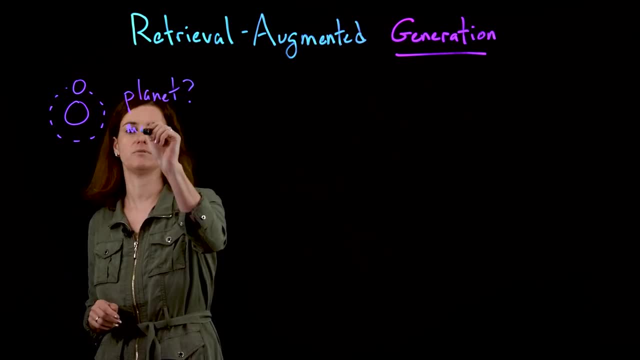 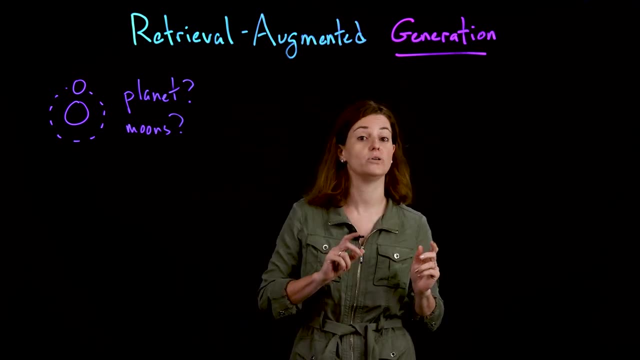 asking me this question. I loved space when I was your age. Of course, that was like 30 years ago, But I know this. I read an article and the article said that it was Jupiter and 88 moons. So that's the answer. Now, actually, there's a couple of things wrong with my answer. 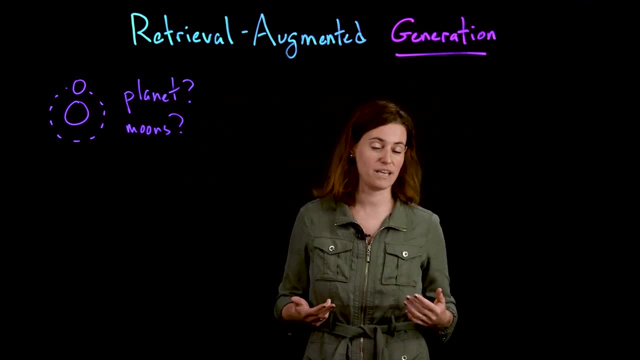 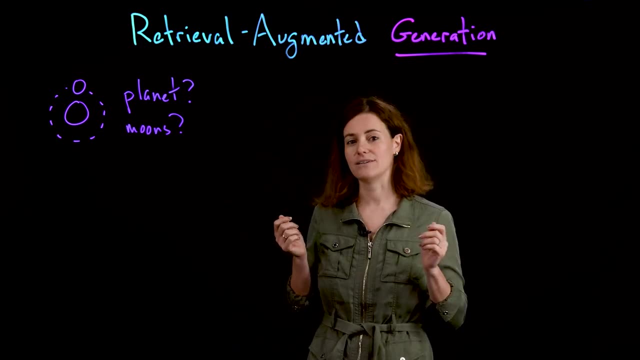 First of all, I have no source to support what I'm saying. So, even though I confidently said I read an article, I know the answer. I'm not sourcing it. I'm giving the answer off the top of my head And also I actually haven't kept up with this for a while and my answer is out of. 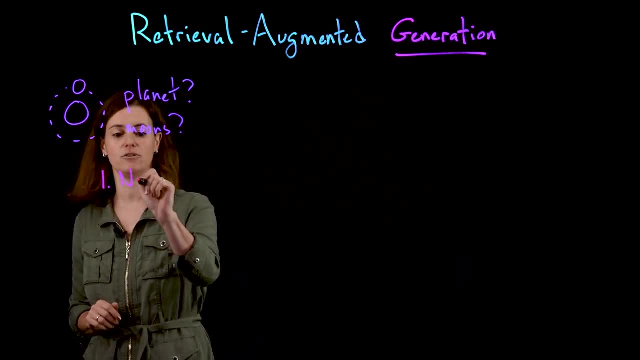 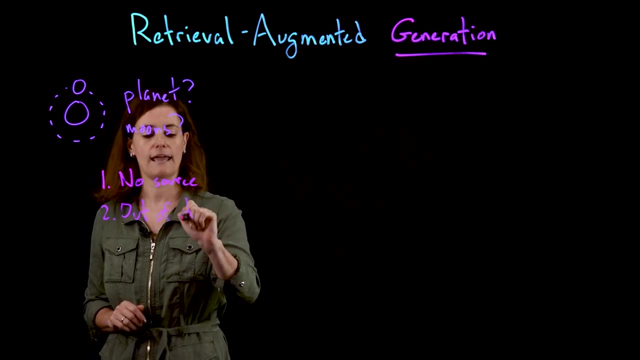 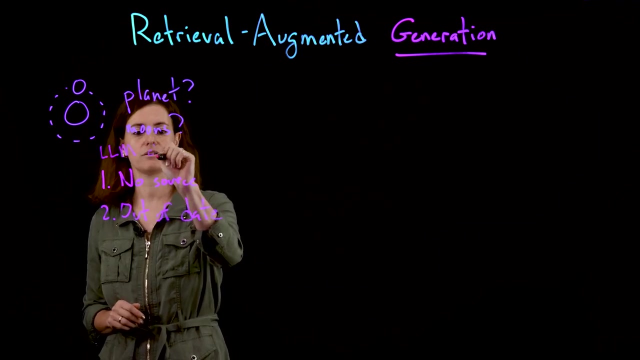 date. So we have two problems here. One is no source, And the second problem is that I am out of date, And these, in fact, are two behaviors that are often observed as problematic when interacting with large language models. They are LLM challenges. Now, what would have happened if I? 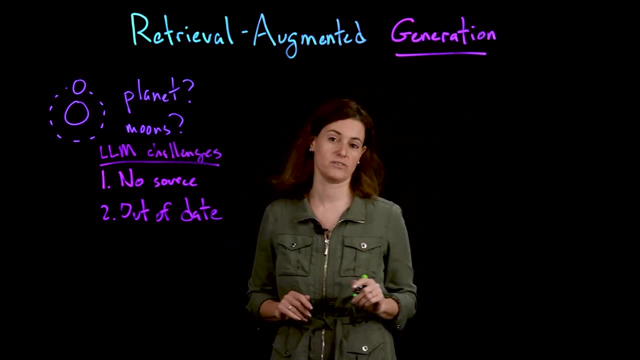 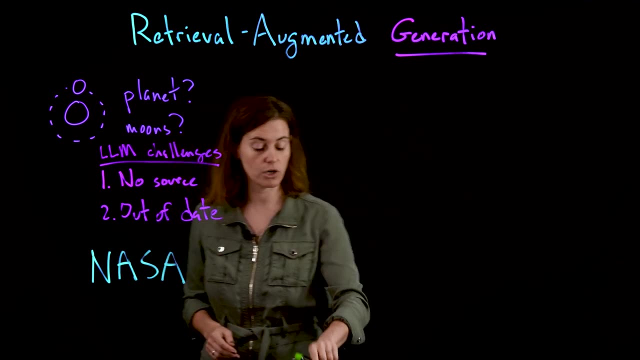 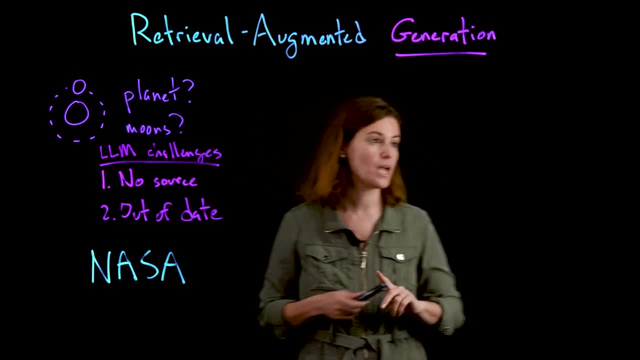 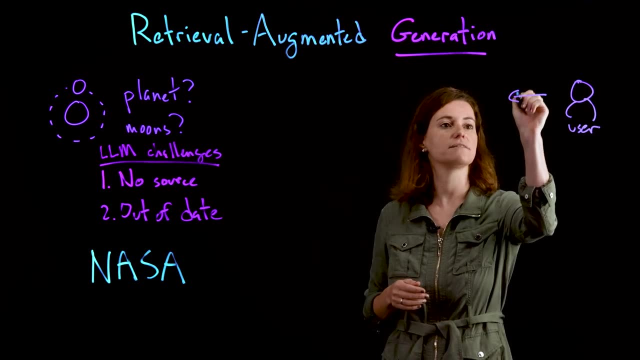 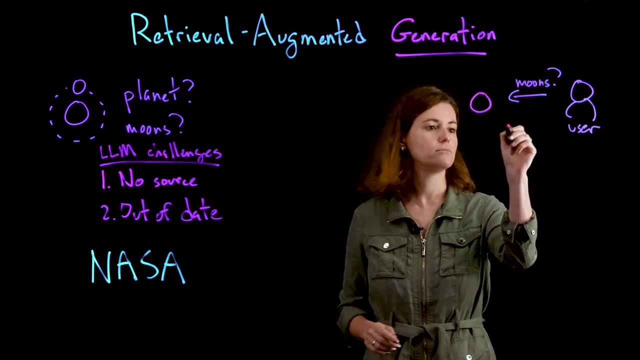 All right. So what does this have to do with large language models? Well, how would a large language model have answered this question? So let's say that I have a user asking this question about moons. A large language model would confidently say okay. 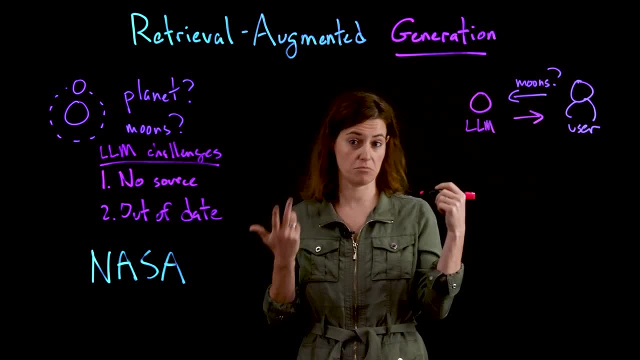 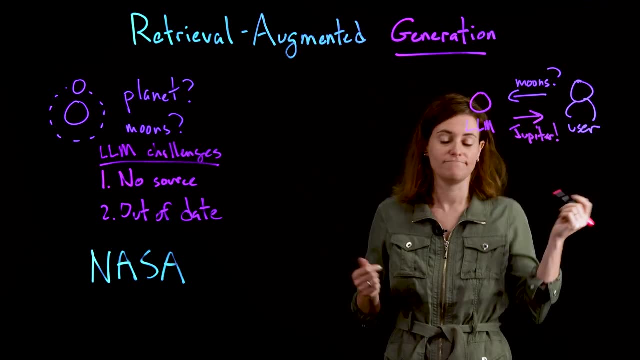 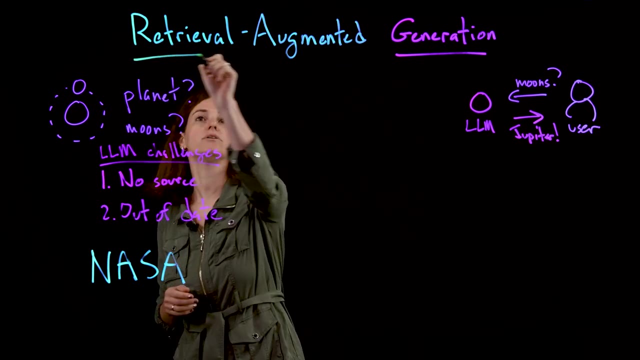 I have been trained And from what I know in my parameters during my training, the answer is Jupiter. The answer is wrong, but you know, we don't know. The large language model was very confident in what it answered. Now, what happens when you add this retriever, retriever, retrieval. 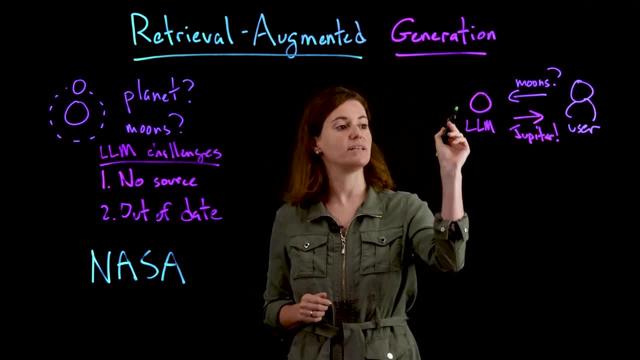 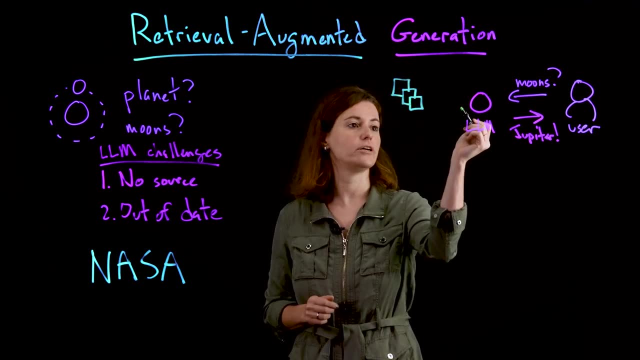 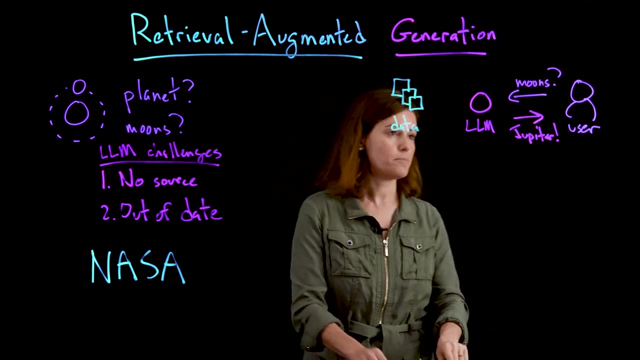 augmented part Here. What does that mean? That means that now, instead of just relying on what the LLM knows, we are adding a content store. This could be open, like the internet. This could be closed, like some collection of documents, collection of policies, whatever. The point, though, now, is that 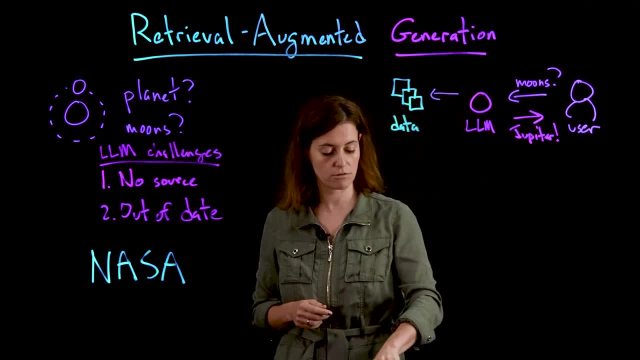 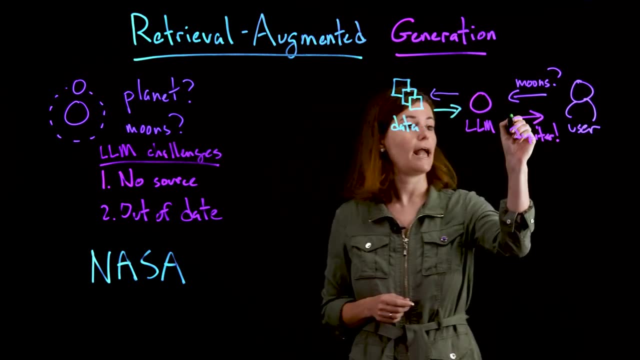 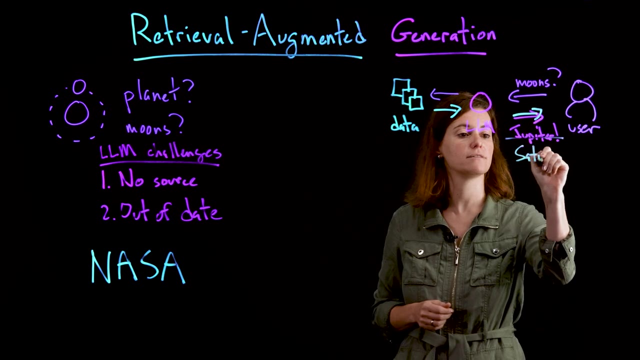 the LLM first goes and talks to the content store and says, hey, can you retrieve from me information that is relevant to what the user's query was? And now this retriever augmented answer: it's not Jupiter anymore. We know that, it is Saturn. 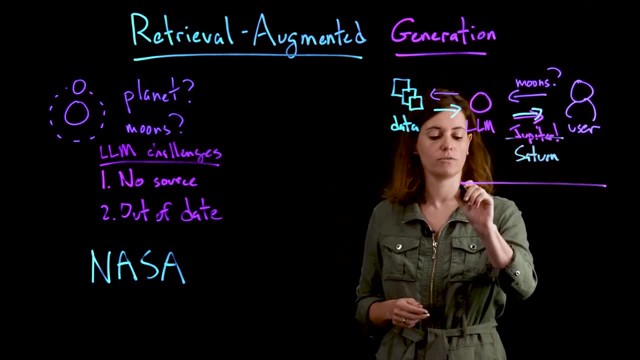 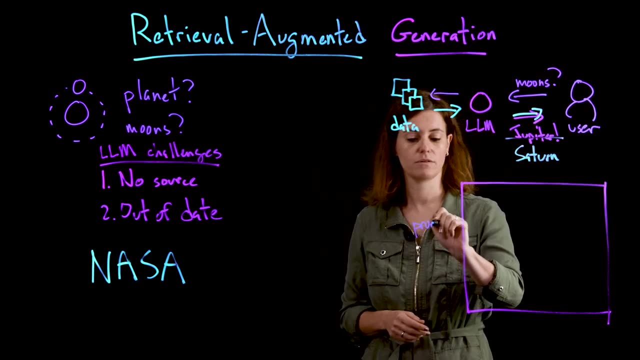 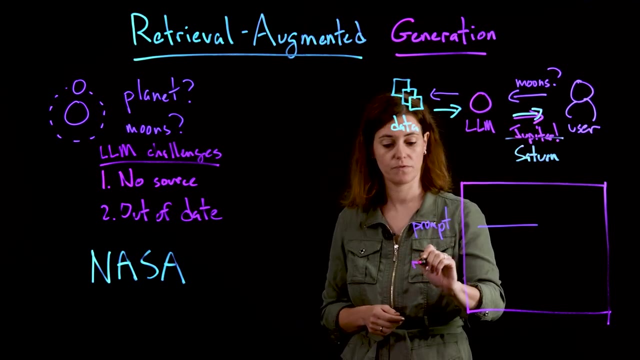 What does this look like? Well, first user prompts the LLM with their question. They say: this is what my question was, And originally, if we're just talking to a generative model, the generative model says: oh okay, I know the response, Here it is. Here's my response. 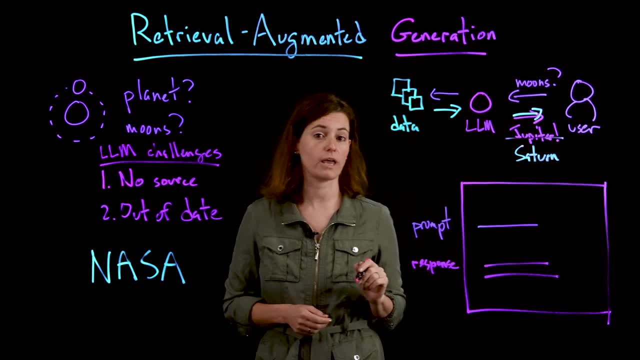 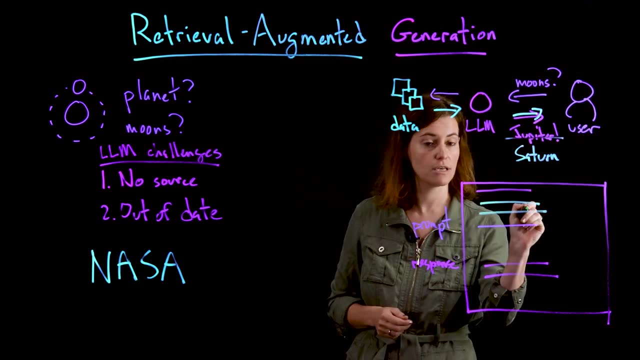 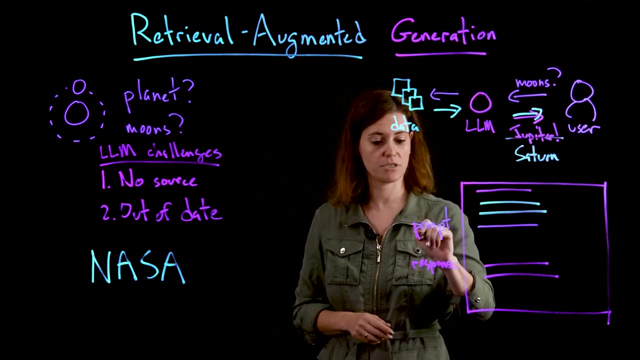 But now in the RAM framework the generative model actually has an instruction that says no, no, no. First go and retrieve relevant content, Combine that with the user's question and only then generate the answer. So the prompt now has three parts: The instruction, 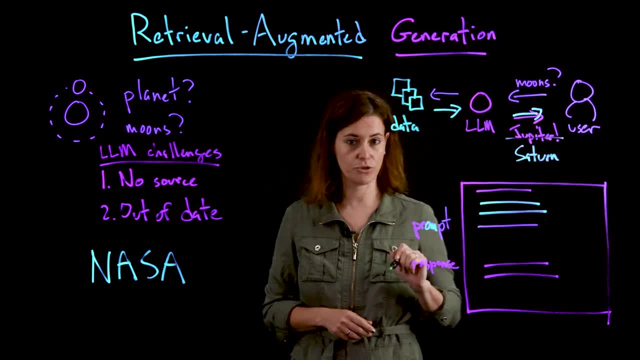 to pay attention to the retrieved content together with the user's question. Now give a response And, in fact, now you can give evidence for why your response is wrong. Now you can give evidence for why your response is wrong And, in fact, now you can give evidence for why your response is. 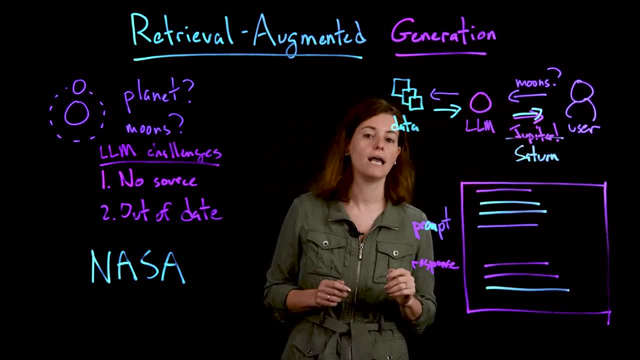 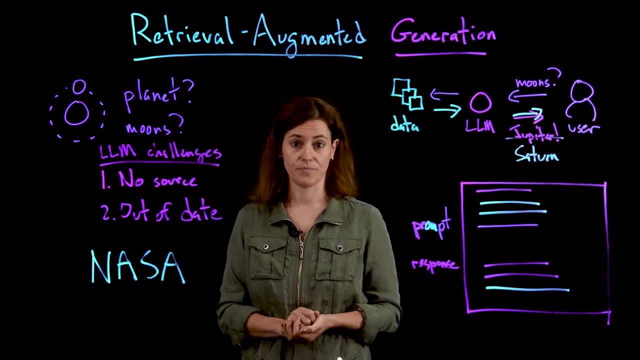 wrong And in fact now you can give evidence for why your response is wrong. So now, hopefully, you can see how does RAG help the two LLM challenges that I had mentioned before. So first of all, I'll start with the out-of-date part Now, instead of having to retrain your model. 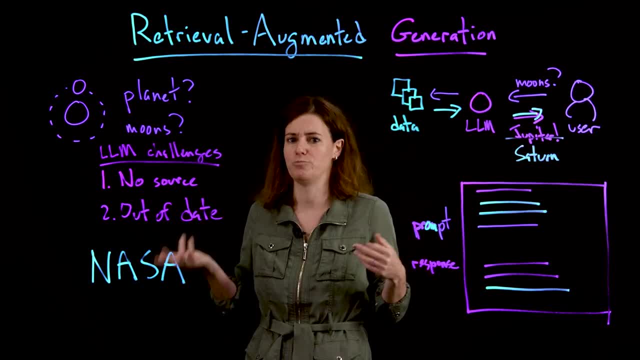 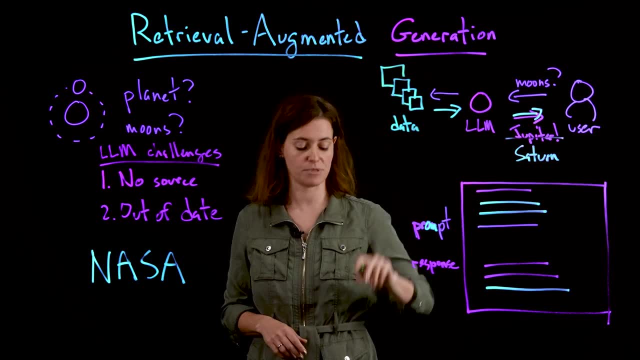 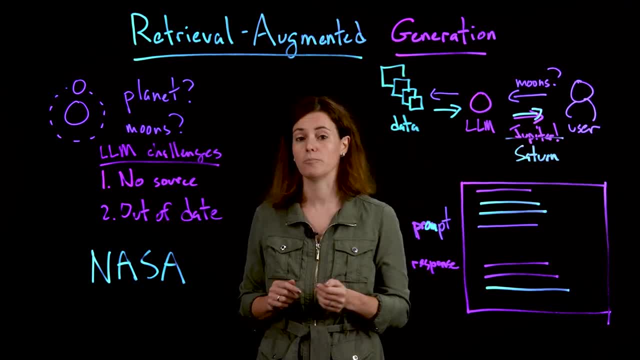 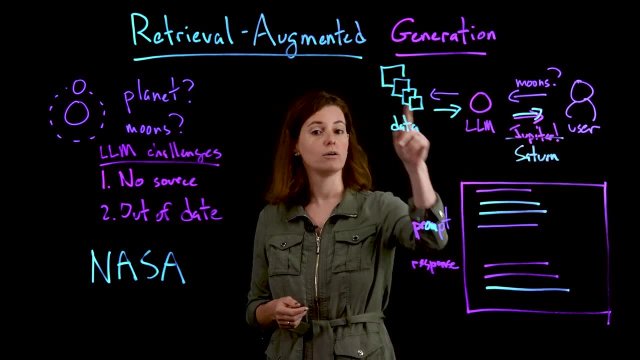 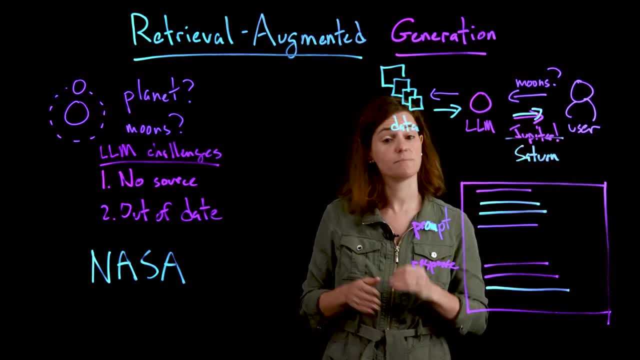 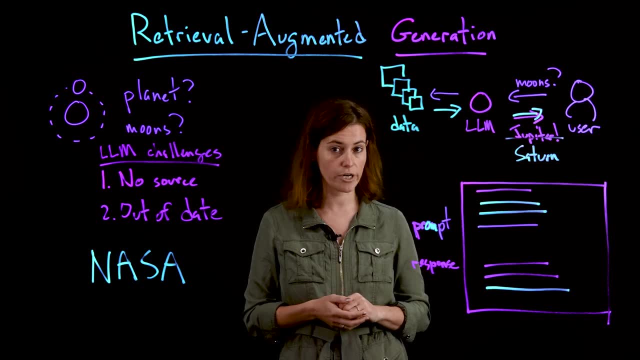 response And, in fact, now being able to give evidence. This makes it less likely to hallucinate or to leak data, because it is less likely to rely only on information that it learned during training. It also allows us to get the model to have a behavior that can be very positive, which 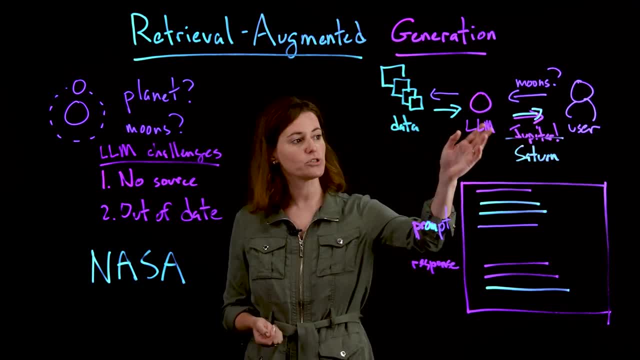 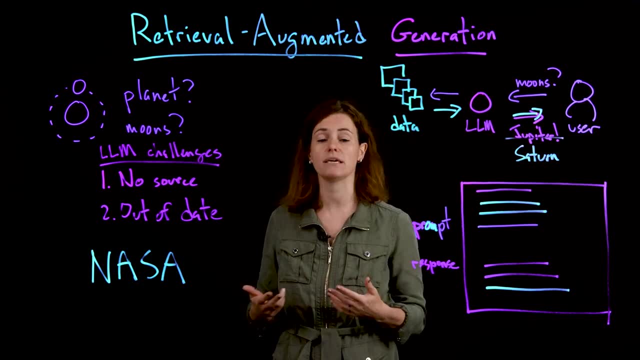 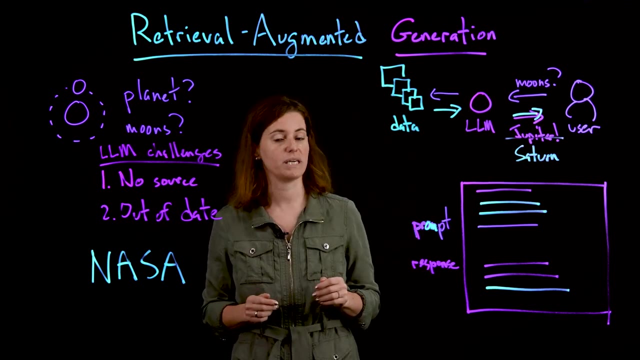 is knowing when to say I don't know. If the user's question cannot be reliably answered based on your data store, the model should say I don't know, instead of making up something that is believable and may mislead the user. this can have a negative effect as well, though, because 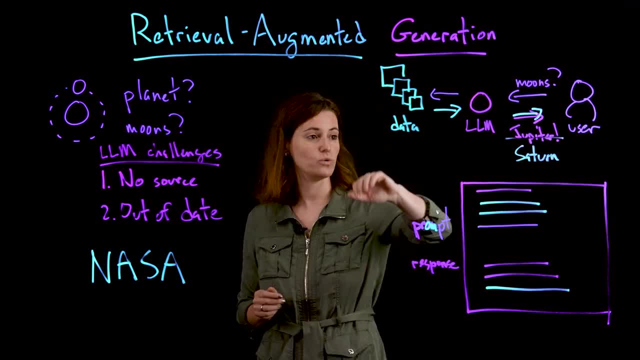 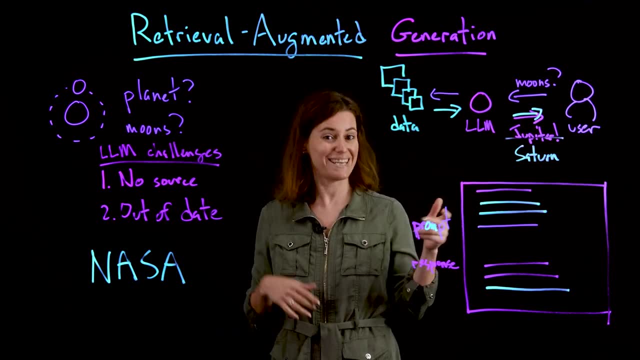 if the retriever is not sufficiently good to give the large language model the best, most highest quality grounding information, then maybe the user's query that is answerable doesn't get an answer. So this is actually why lots of folks, including many of us here at IBM, are 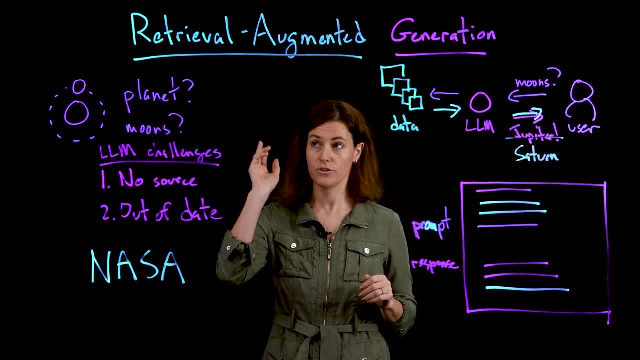 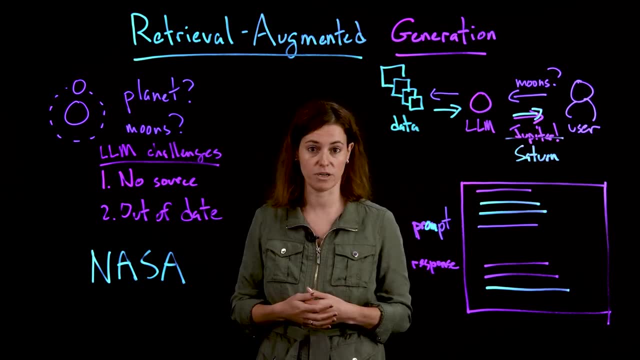 working the problem on both sides. We are both working to improve the retriever, to give the large language model the best quality data on which to ground its response, and also the generative part, so that the LLM can give the richest best response. finally, to 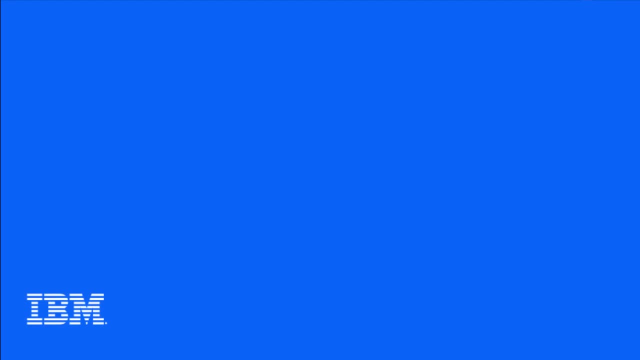 the user when it generates the answer. Thank you for learning more about RAG and like and subscribe to chat. Bye for now, Thank you.